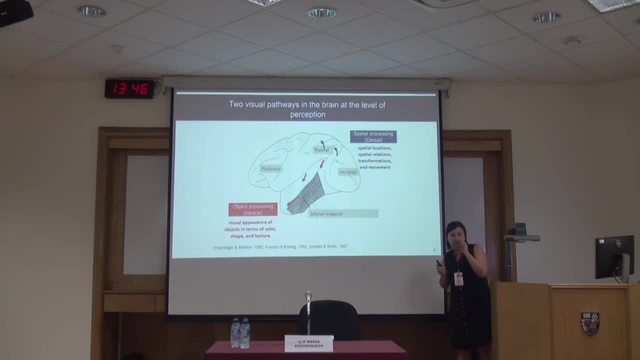 Spatial relations and spatial locations. So this is two different visual systems. A person is able to perceive spatial locations, not able to perceive appearances of individual objects, and vice versa. Similar dissociation was found in visualization, visual imagery. People with damage in this object processing ventral pathway were able to visualize spatial relations. 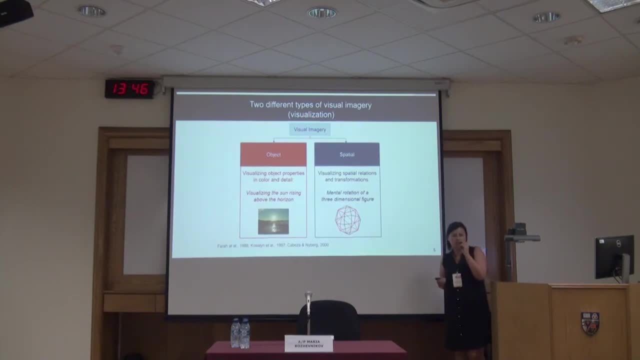 but were not able to visualize individual objects In terms of their color or shape and vice versa. So this is two types of visualization. They're independent And actually it's clear, visualizing the sun rising above the horizon. It's a very different types of visualization: that solving geometrical problem or mentally rotating complex geometrical figure. 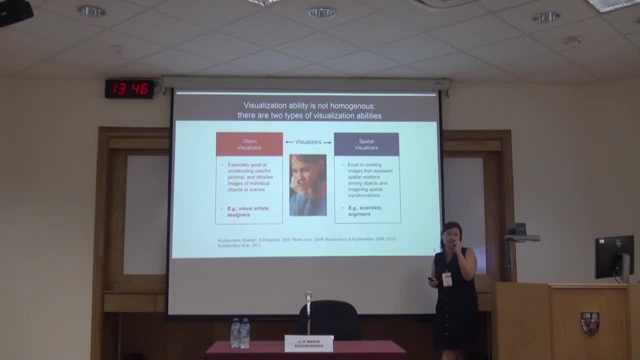 So my research is about individual differences in these types of visualization And what I show. I show that there are two different types of people: Object visualizers who hide in object visualization ability, And I'll show that these are visual artists and designers. 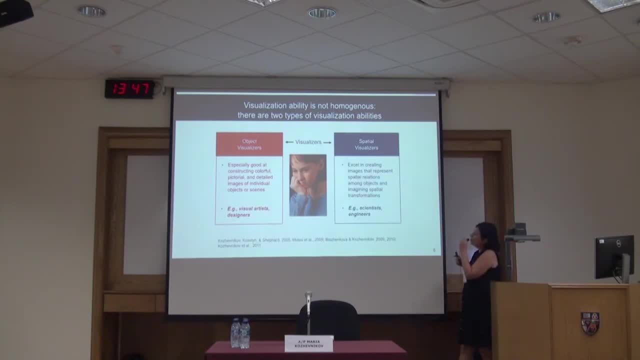 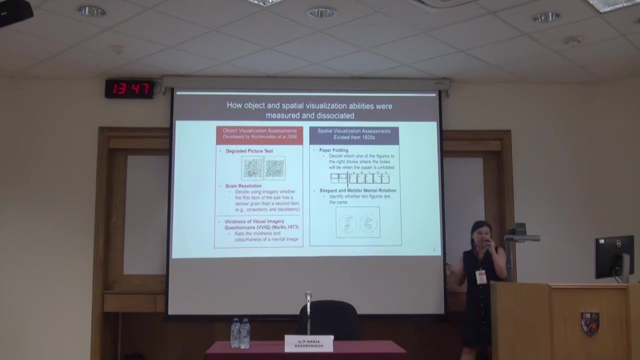 And spatial visualizers. These are people who hide in spatial visualization ability, Such as scientists or engineers. So how to measure disabilities For spatial ability? it's not spatial visualization ability. It's not that difficult, because the tests were designed 100 years ago. 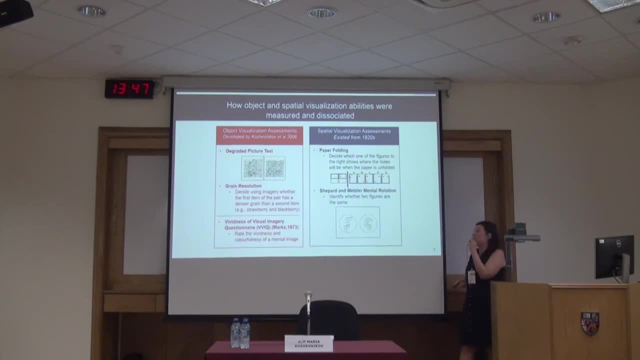 And they were used in army for personal selection in medical school. So this is classical spatial visualization ability test. Paper folding: Decide which one of the figures to the right shows where the holes will be when the paper is unfolded. And the answer is C. 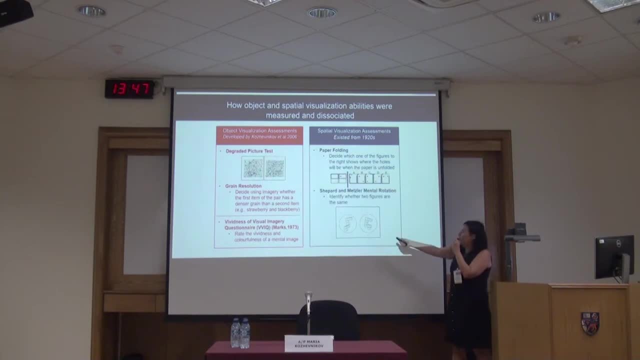 But this is a simple one. The real one much more complex. Or to mentally rotate two figures and to identify where there's the same or mirror reversed. So this is spatial. As for object visualization test, it's very new. We only know from late 80s that this type of visualization is different. 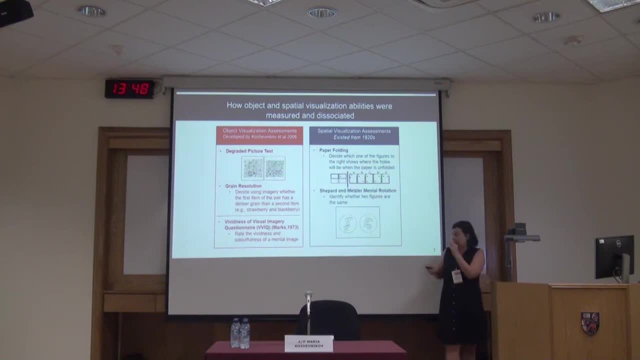 So our lab was designing this test for years, And the first one which measured shape imagery. This is object visualization imagery And this is a test to identify figures hidden in the noisy pictures And if you can see any particular images, If anyone can see something on screen. 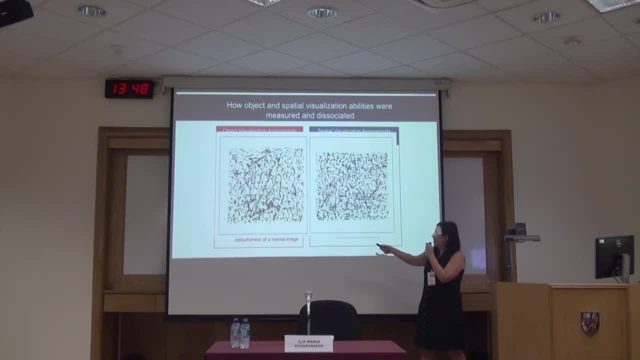 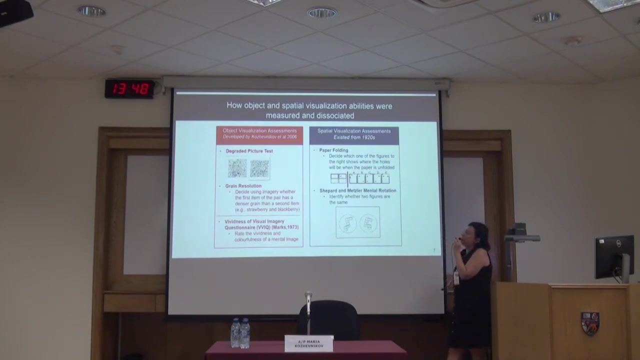 This is the left, This is umbrella Here and here is scissors. So we measure accuracy and response time. And there was two other grain resolution. This side is an imager where the first item of the pair has a denser grain than the second item. 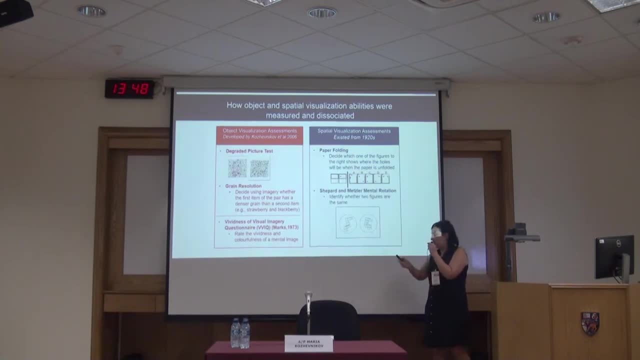 And strawberry has denser grains than blackberry And this is classical vividness of visual imagery questionnaire Which was developed Before in 1973. The vividness of colorfulness of mental image. So, by giving all these tests, what we found? 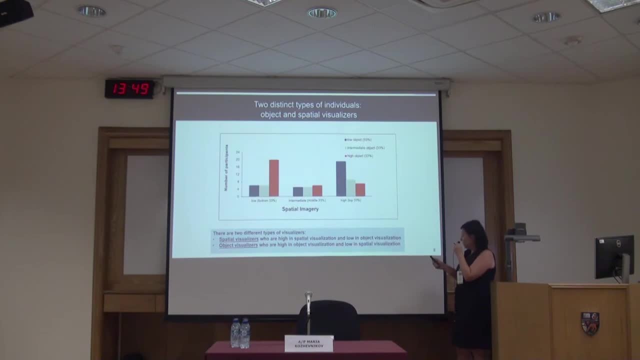 This is my previous study. We found that if to categorize people as low spatial, intermediate spatial, high spatial, into three groups And then to categorize them as low object imagery, intermediate object imagery and high object imagery, You can see this by model distribution. 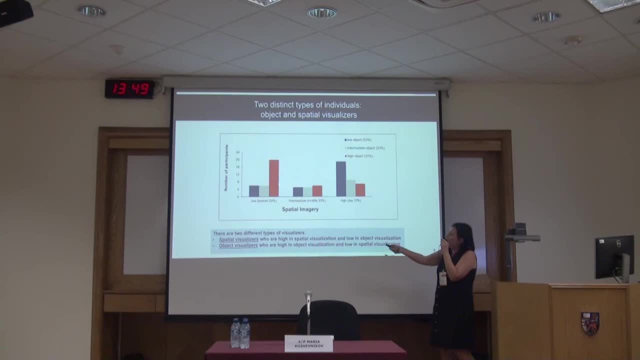 Most low spatial imagery people. They are high object visualization people. Most people with high spatial ability- They are low object visualization people. So there is clearly some tradeoff between these two abilities. And people who have high spatial visualization ability Clearly do not have, on average, high object visualization ability. 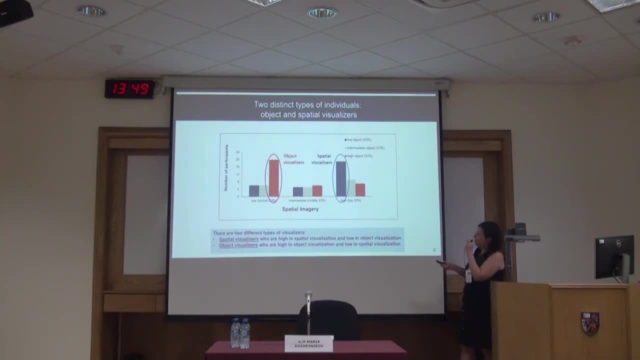 And vice versa. So now I'll show you some neural evidence That this is not neural, This is developmental evidence, And this data is for children Starting from 11 years old to adults, 40 years old, To show how different is two visualization ability. 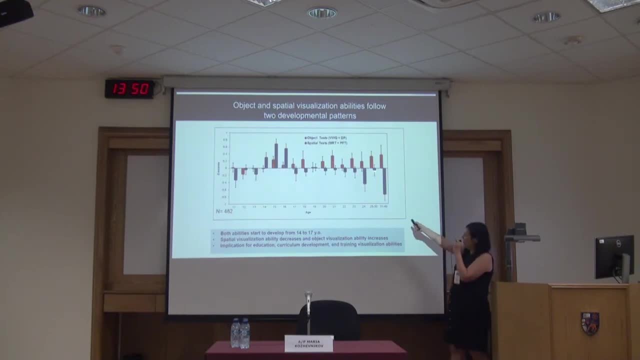 So zero means average in the sample. It doesn't mean zero ability. Blue means spatial ability, Red is object visualization ability And, as you can see, spatial visualization ability. They both developed around 14, 17 years old, But spatial visualization ability peaks during this critical period. 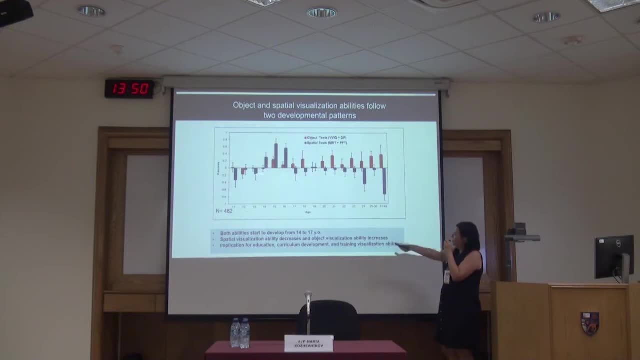 And then it declines While object visualization ability develops across the lifespan. So these data have quite significant implications for education and curriculum development, Because it looks like science better to teach during these years To support the development of spatial visualization ability, And art can be taught anytime during the school. 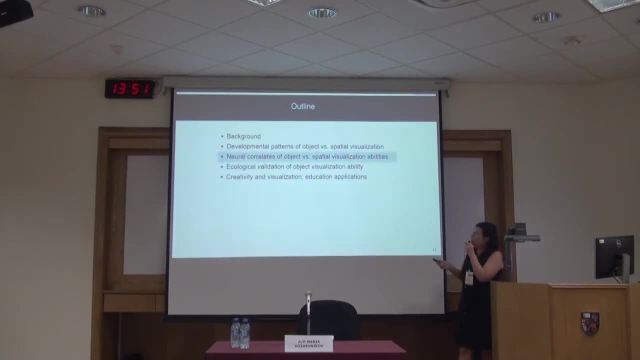 So now I'll show evidence about neural Neural evidence that these two abilities are very different And draw on different neural resources. So previous study shows that spatial visualization- Low spatial visualization- people Have higher activation in spatial dorsal processing pathway And also frontal attentional areas. 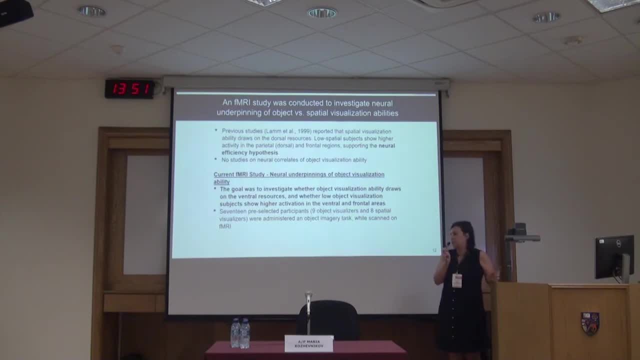 Because it's difficult for them to process spatial information. So this is called neural efficiency hypothesis: The less ability you have, The higher activation you show in this task specific area. So now we wanted to show the same for object visualization ability. Now we were looking at ventral pathway. 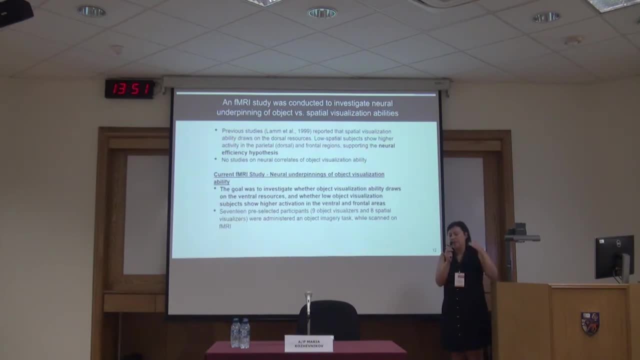 And to show that object visualizers: They have low activation And low. object visualizers Have high activation in ventral pathway And low activation in ventral and frontal pathways. So we used 17 people, 9 object visualizers And 8 spatial visualizers. 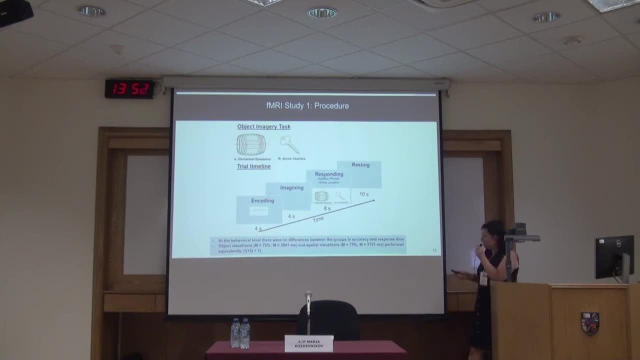 And we scanned them at MRI. This is the task. This is object visualization task. People presented with images For 4 seconds, Then they asked to visualize. Then they asked the question: Was there specific properties Such as arrow junction or horizontal symmetry? 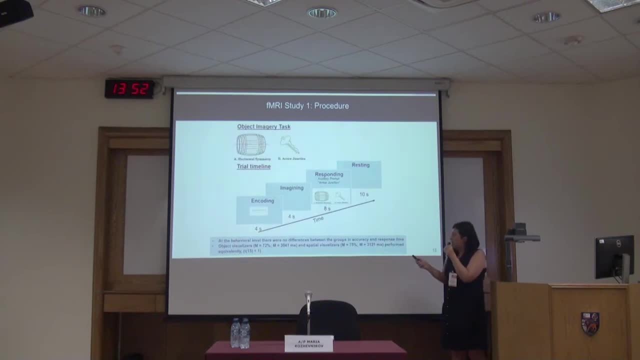 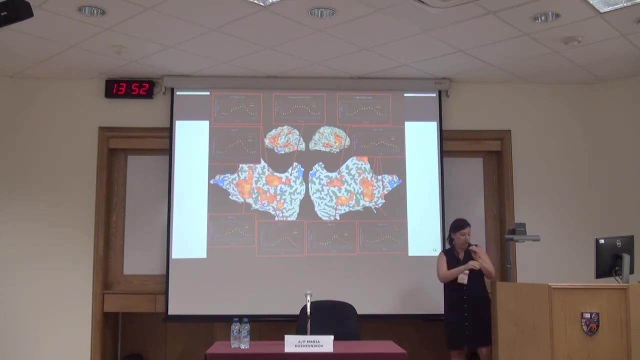 Was an original image- And then resting period, And here I'll just explain very briefly this result. So this is flat end brain And you look on this brain from above. So this is ventral area, Area responsible for processing. This is left. 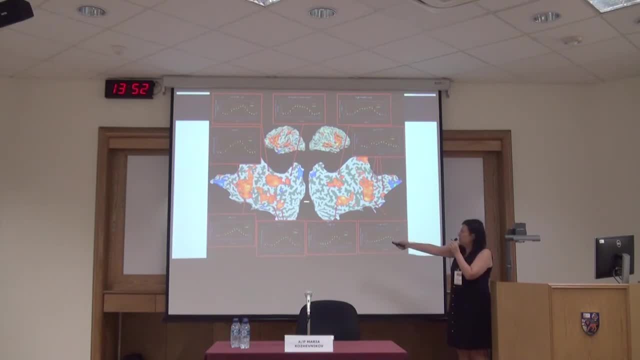 Right brain and left brain. This is area responsible for processing object information, So responsible for object perception and visualization. So and if? to look How two groups perform This area? So right, here is spatial visualizer That shows Significantly high activation than object visualizer in this area. 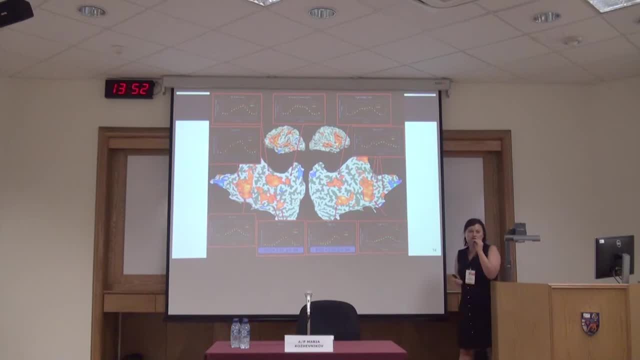 Which means that it's really hard for them to process object visualization task. So these high spatial people apparently do not have enough resources To remember these objects, So they recruit way more this area than object visualizers And similar. So similar- This is frontal areas. 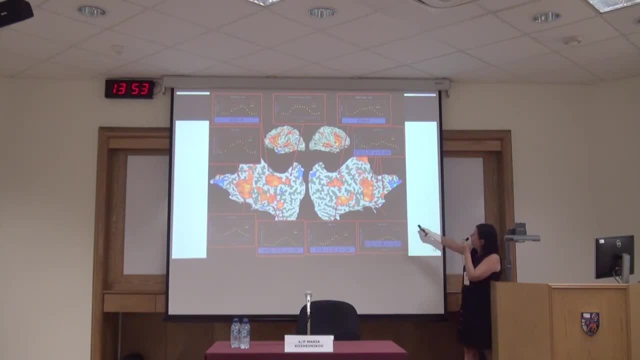 And in frontal areas, Again, Object visualizers Have significantly higher Low activations than spatial visualizers, Which means that spatial people They recruit more frontal resources to perform the task. So, and in conclusion, In neural level, We can see that object visualization ability draws on very different pool of neural resources. 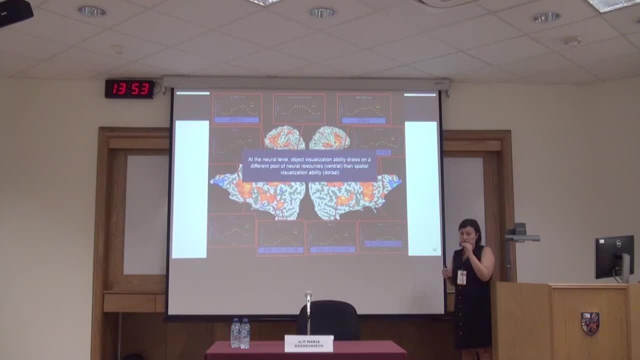 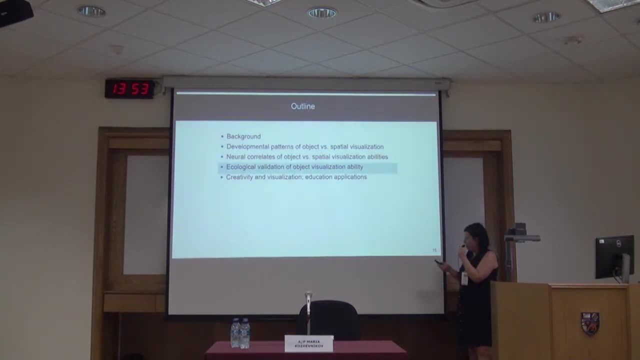 Than spatial visualization ability. They definitely clearly two very different abilities. Okay, So now I'll show some studies Which argue for ecological validity of object visualization. Now we know that spatial ability, Spatial visualization, is very important for science and engineering. But where is that this object visualization ability important? 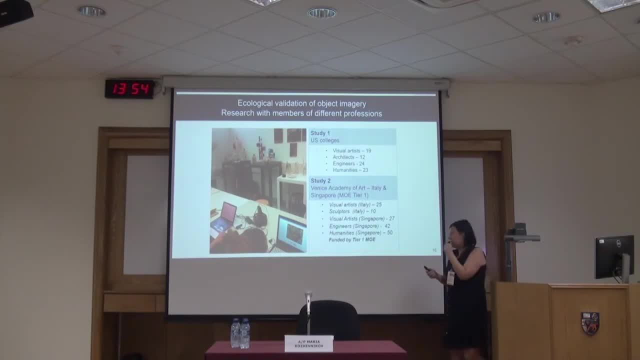 So our hypothesis was: It's important in art And I'll show two studies. The first study was done in US colleges- This is faculty professors who participated in the study, And we were interested in comparison, their object and spatial visualization skills. And second study was done here in Singapore. 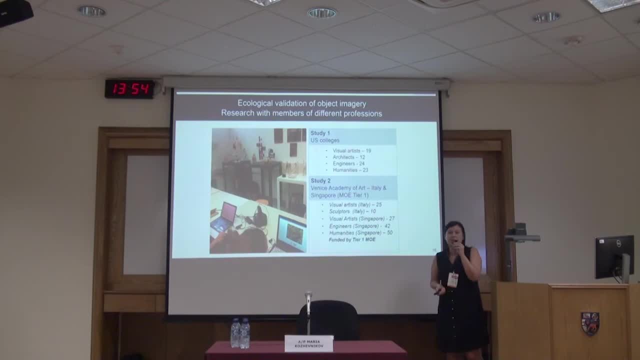 And also in Italy. We studied Italian artist and Singaporean artist And we were interested to compare their object visualization skills. And also in the second study We were interested to compare different, more fine grained sub components of object visualization. This is the first study. 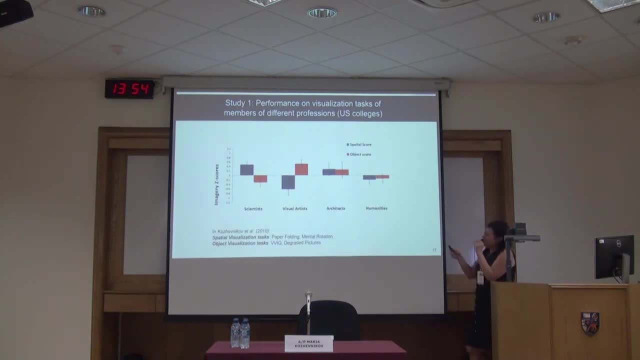 So this is. It was done quite long time ago, But I just wanted to show Fine study, Fine study. So again, This is zero means average in the sample. Blue: This is spatial scores. Red: This is object scores. 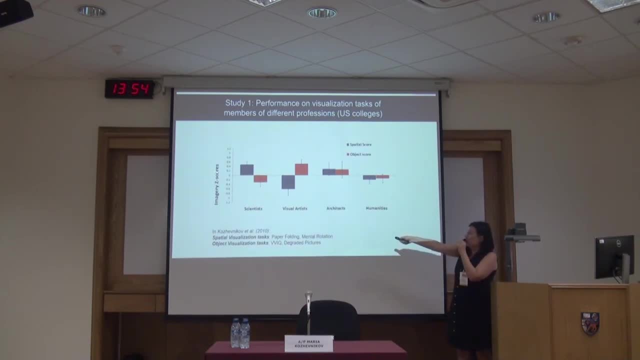 Scientists have highest average scores on spatial ability, But below average scores on object visualization ability. It's vice versa. for visual artists. It's not very clear for architects. There is huge standard deviation And it's about average for humanities, So definitely. 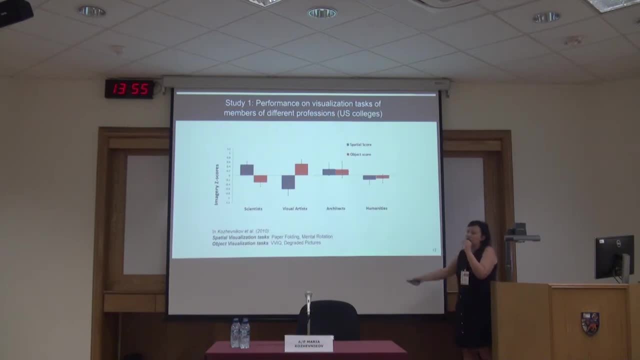 There is again this trade off: Scientists who develop high spatial visualization ability Somehow underdevelop object visualization, And vice versa for visual artists. So- and this is study, The second study, Here we had way more tasks on object visualization This one. 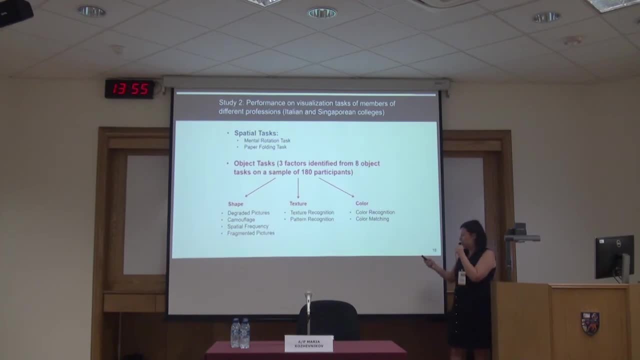 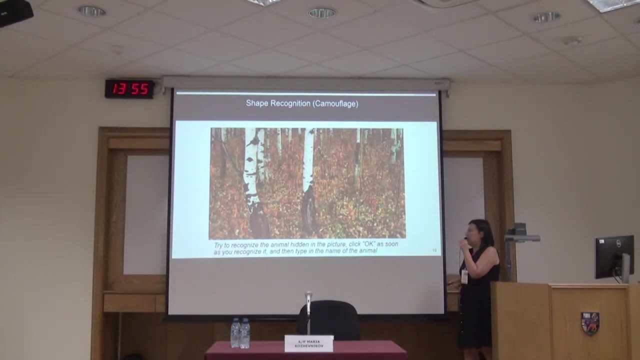 Okay, So this is shape imagery, Texture imagery And color imagery, So different sub components And this is task on shape visualization To recognize the animal hidden in the picture. And there is an animal here And I don't know if you can see. 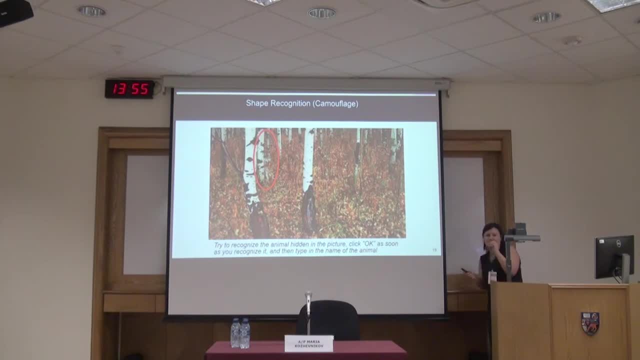 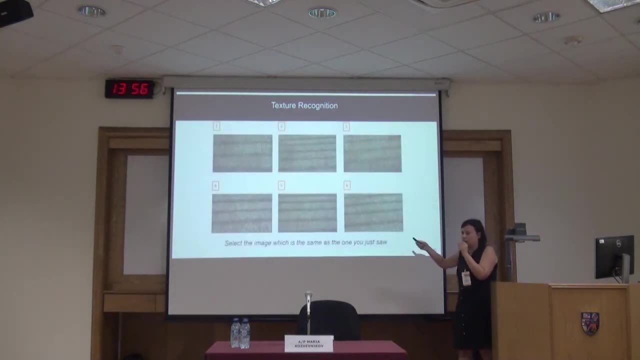 The animal is here, It's wolf. So this is shape recognition: To recognize shape in hidden environments. This is texture recognition Image shown for few seconds, And then you need to select the image which is the same as the one you just saw. 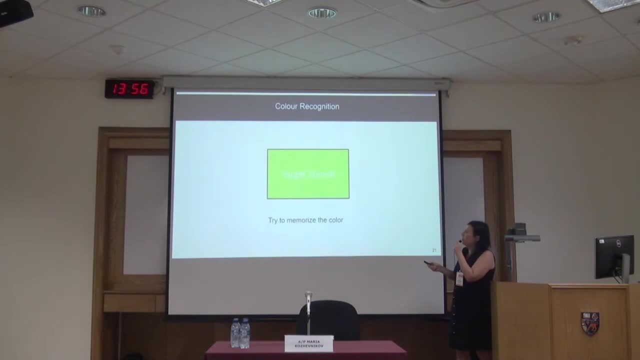 And this was image number two, Similar for color. What color was just shown? And the correct answer is that one. So usually this test is very easy for visual artists. They are more difficult for scientists. So if somebody experience difficulties, I mean really more scientific direction. 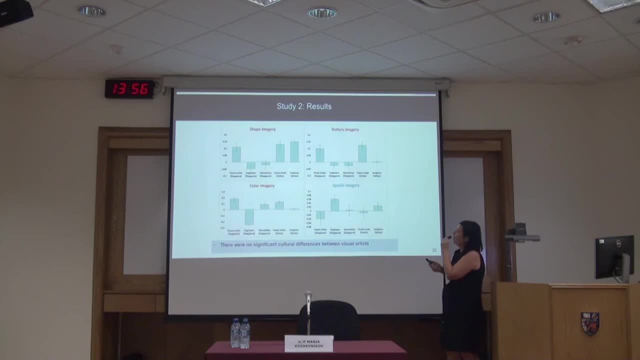 Okay, So this is the results. This is the results across countries And across people of different professions. So, first of all, We found no differences between Italian and visual artists on any of these tasks. On any of them, There were no significant difference. 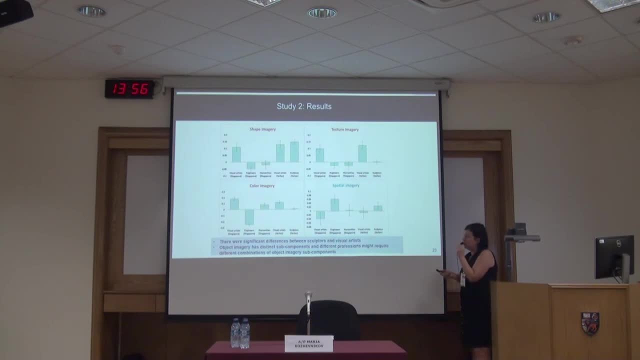 But we did find difference between people of different professions. So sculptors, Sculptors were no different from visual artists on shape imagery- This is, find an animal. They were no different, But they were significantly different on texture imagery. Apparently, sculptors do not have texture imagery. 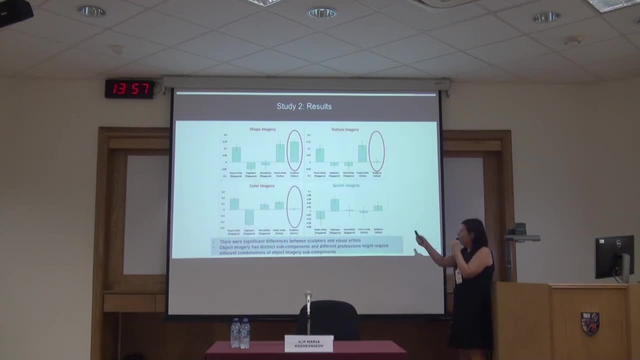 They also do not have color imagery, In contrast to visual artists, But they have quite high spatial ability, Almost similar to engineers. So, In conclusion, Object visualization has distinct sub-components And different professions may require different combination of object imagery capabilities. 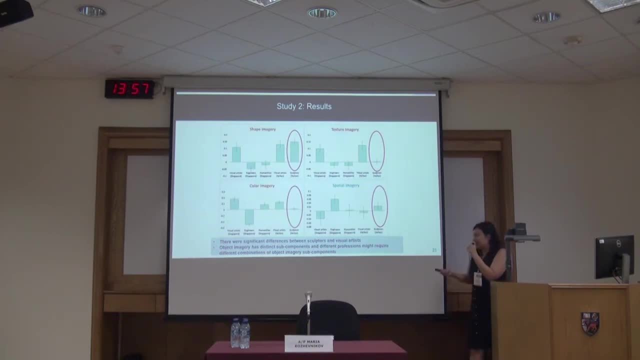 So we need to study this further, Because architecture is another example. We don't know what kind of combination architecture require: Sculptures and so on. Okay, And the last study is about creativity and visualization. So creativity We already heard from professor Opstein. 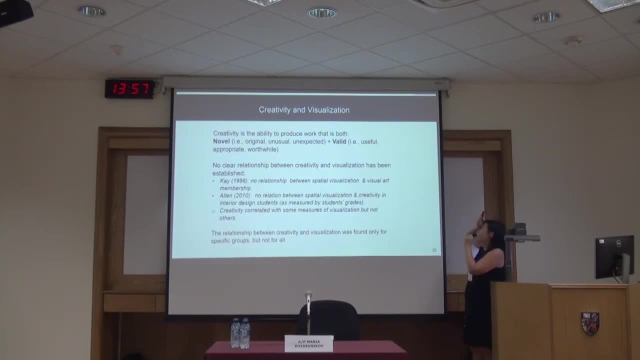 Very difficult to measure- A lot of tests- And very difficult to define operationally. So this is ability to produce work that is novel and valid, But- And it's clear, intuitively, it should correlate with imagination and visualization. But Very difficult to show any relation between visualization and creativity. 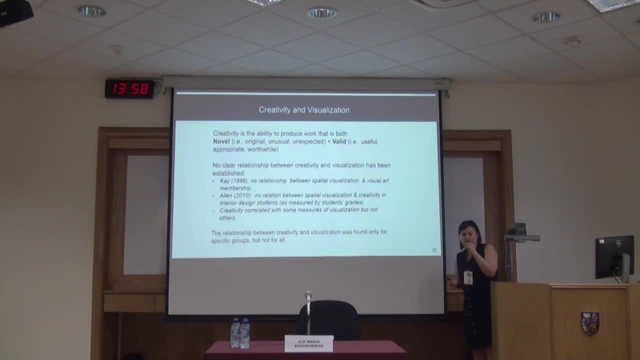 There were many studies But the relation was not established. So for some groups There is correlation, For other groups there is no correlation. There are many different tests on creativity. They are not very well validated, So It was completely So there is no clear relation. 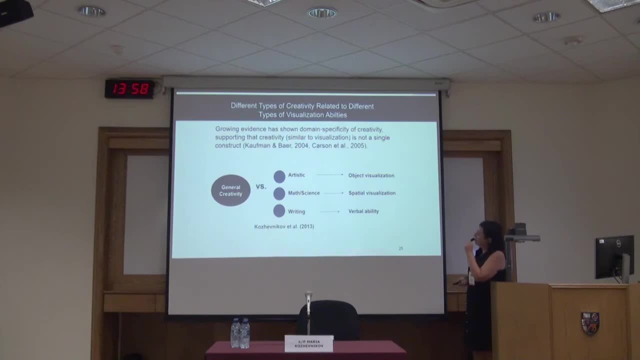 So, based on my previous research on object and spatial visualization, I just separated, And based on recent research about creativity As domain specific, I separated scientists versus artists And then I separated object visualization test from spatial visualization test. So here you can see clear correlation. 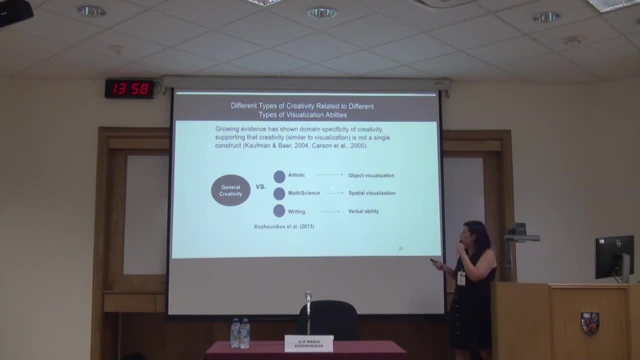 Artistic creativity and test that measure artistic creativity, as well as self reports. They correlate clearly and highly with object visualization, While scientific creativity correlates highly with spatial visualization. So Again, It means that there are very different types of creativity, Very different type of visualization. 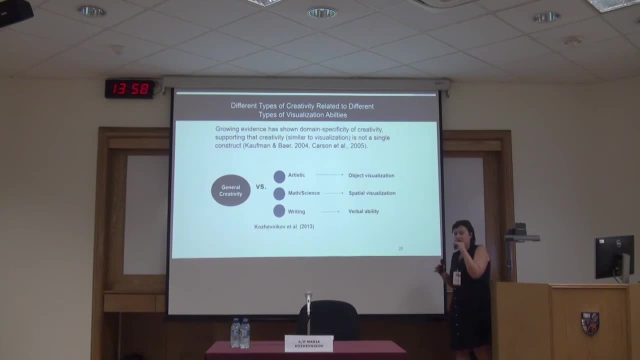 There is even trade off between them. A person creative in art Probably will not be very creative in science, And vice versa, So you should take this into account while designing curriculums. Like overall approach To develop holistic thinking Is not working for scientists. 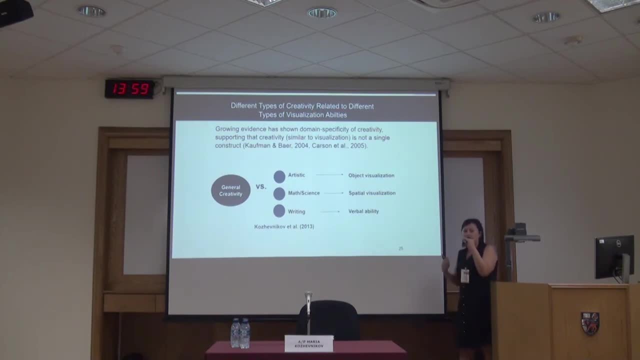 It might work for artists, So all this should be taken into account. So This is new grant In which We are now planning to investigate development of different types of creativity And their corresponding visualization In children of 13, 16 years old. 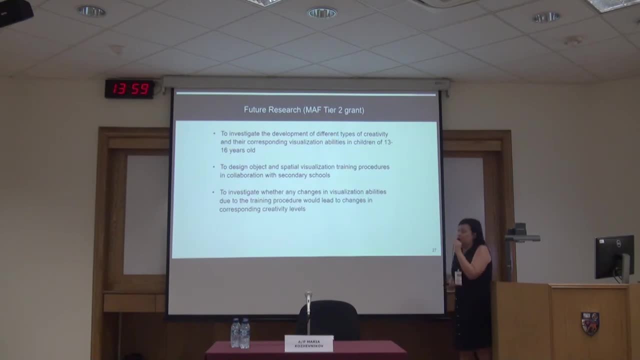 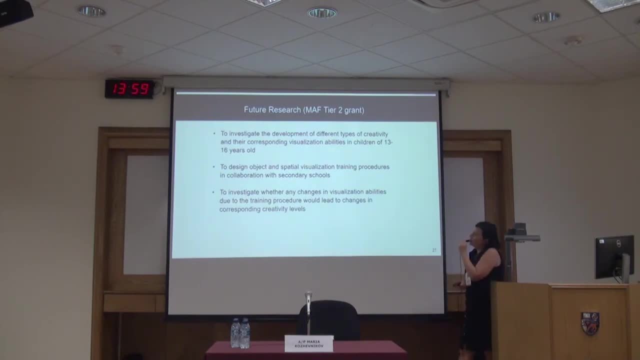 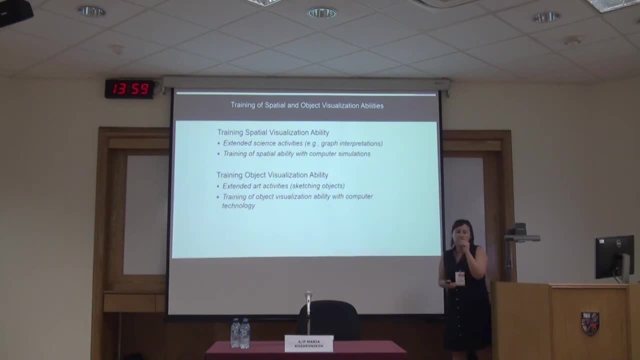 To train spatial Or object visualization ability, And so far And again, Not about Objects, about special visualization- is Extremely difficult to Train special visualization And usually all the training is presented Monday. I mean on one task. but when you try to give another spatial task, people don't know better. 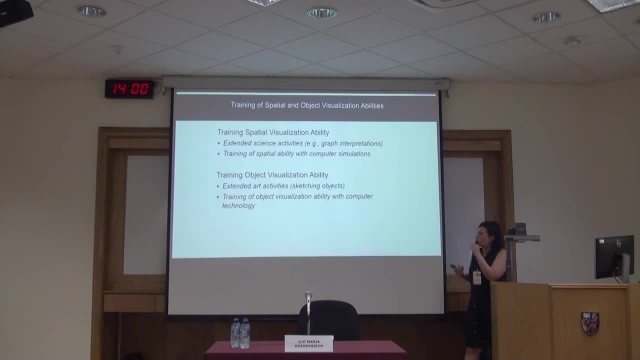 So the question here in this research is, first of all, how to train spatial visualisation ability and second, how this training will affect object visualisation ability, Because we don't know. now there is a lot of spatial training workshop everywhere in the world because they want to improve scores on science and science and engineering we 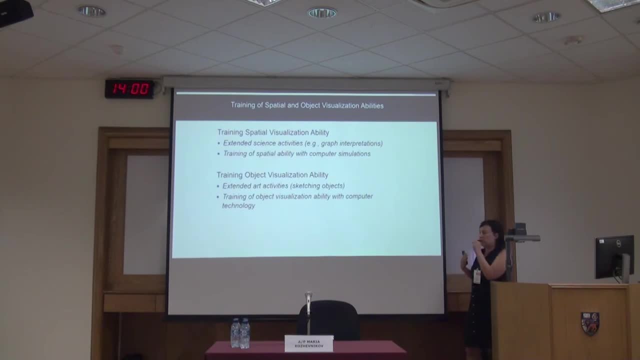 don't know how they will affect object visualisation ability because of this trade-off that might actually impede the development of object visualisation. So in this project we want to take this also into account. Just a few more slides about how to train spatial visualisation and it appears that 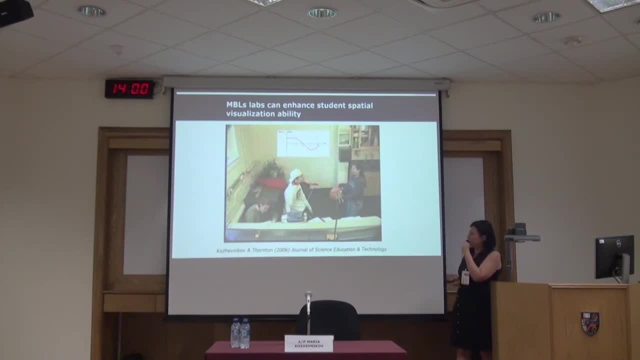 training which used multiple representation, helped to train spatial visualisation ability. This was MPL curriculum- very old studies, but what we found? we found that MPL is a very useful tool. When you throw a ball or you move the object, a graph appears in real time on the screen. 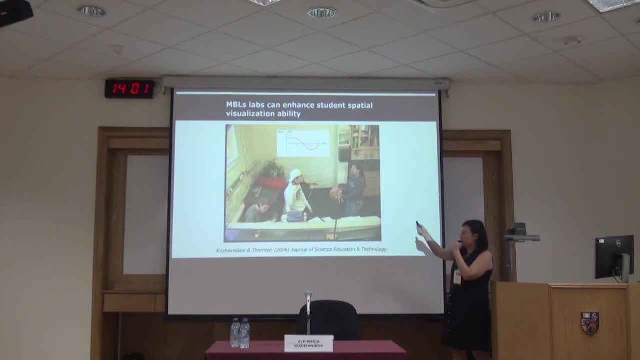 so people can relate this pictorial representation of moving objects with real schematical representation. This curriculum helped to develop the spatial visualisation ability to some extent. this is control group. this is high spatial but medium spatial. people did develop the spatial visualisation ability after this intervention, after this course. 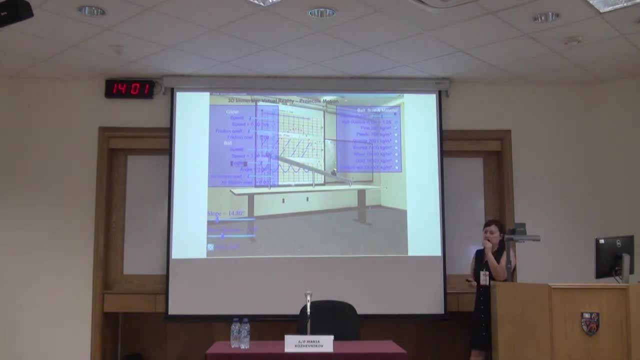 So what we are doing now here at the US? we are developing virtual reality, which is a tool which combines multiple representation, including pictorial movement of objects. there are graphs which actually impose not only in real time, but also in space. you. 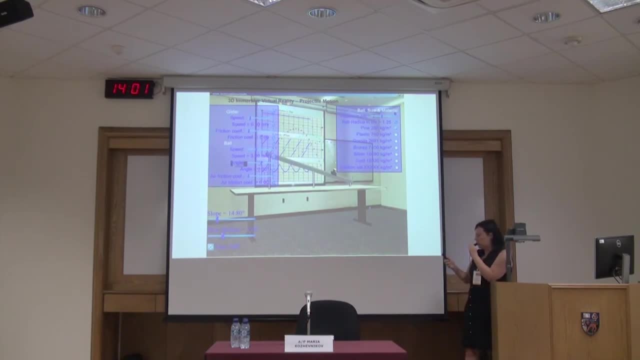 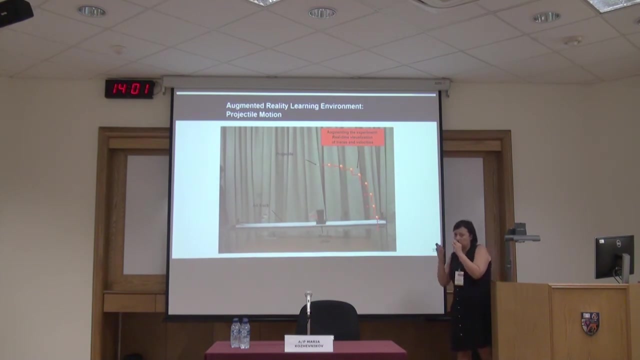 can move the graphs. you can see the graphs. you can see how they appear as object moves. So now we investigate how this curriculum can help to improve students' spatial visualisation skills. Okay, so this is augmented reality, the same. how all this interposition of schematic and 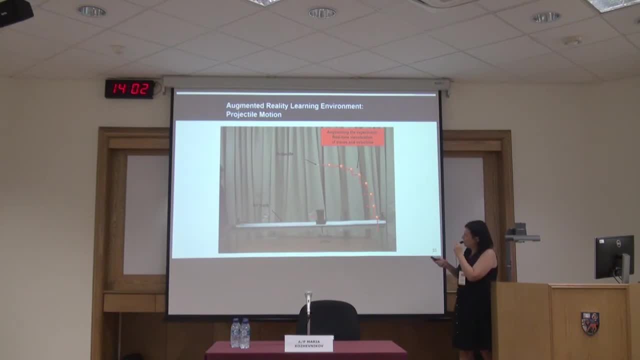 pictorial representation can help to improve spatial visualisation. Okay, so this is augmented reality. the same how all this interposition of schematic and pictorial representation can help to improve spatial visualisation. Okay, so this is augmented reality. the same how all this interposition of schematic and 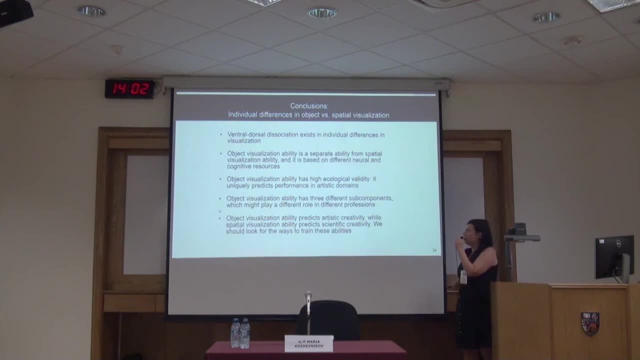 pictorial representation can help to improve spatial visualisation. Okay, this is just conclusion. definitely, Object visualisation ability is separates ability from spatial visualisation. Draws from different types of neural and cognitive resources. has high ecological validity. has three different sub-components- shape, colour and texture- which might play different. 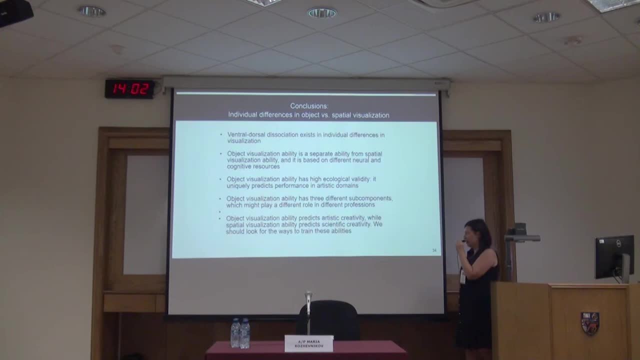 role in different profession, And object visualisation predicts significant artistic creativity, while spatial predicts creativity in science. Have a good day. So in the game, we should look for the ways to train disabilities, investigate how development of one can impede the other. 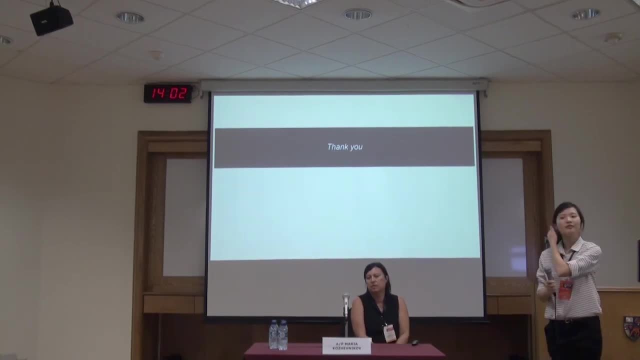 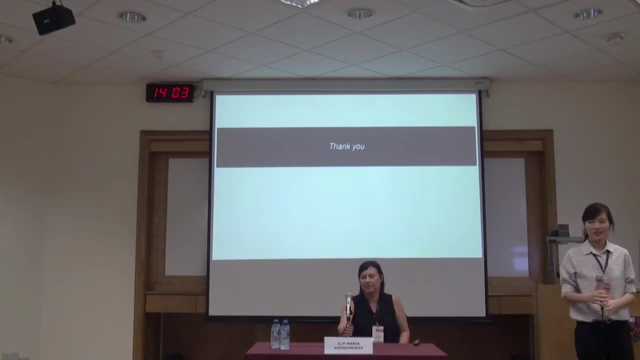 Alright questions. This is fascinating research. I love it And I think I want to ask a question about the two cultures and about the developmental data that you have. So this whole idea that the arts and the sciences are completely different subjects and that people are naturally inclined to go towards one or the other? 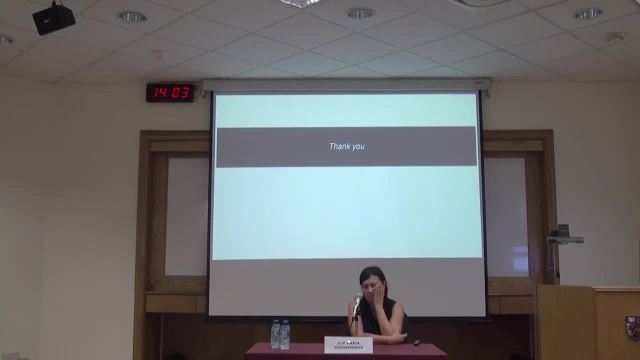 and that once we specialise, that becomes the niche that we become experts in. When I look at your developmental data, we see this bloom in the 13 to 16 year olds, where both forms of visual expertise are really high, and then one has a little dip and then increases. 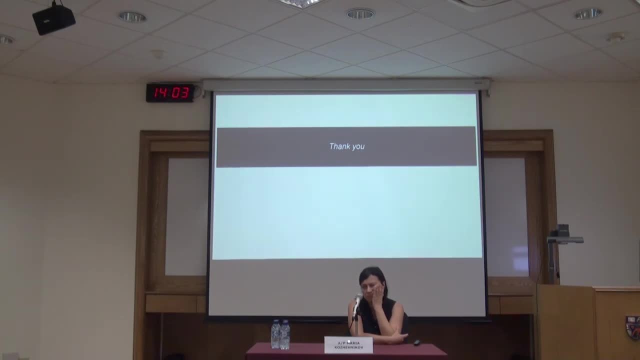 and the other has a little dip and continues to decrease for the people in the developmental data you showed. What that suggests to me is that the specialisation, this trade-off that you're talking about, may not be neurologically mandated. it may be socio-culturally governed, by the expectation that you either take science studies or arts. 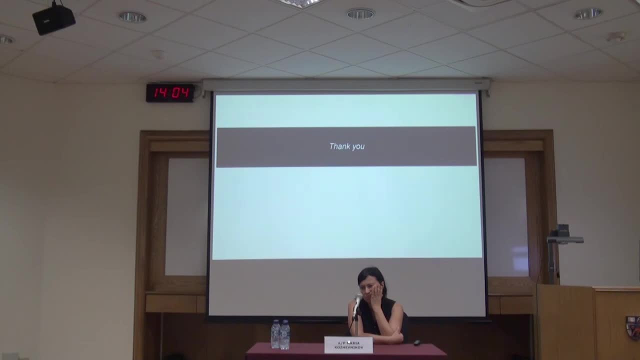 So I'm kind of interested in your thoughts about how that might relate to the kind of data that you have And the architects. You seem to have both Developmental data. so I did developmental study where our kids were. We took the kids six, seven years old and another group 12, 13 years old and another group, you know, up to university and graduate studies. 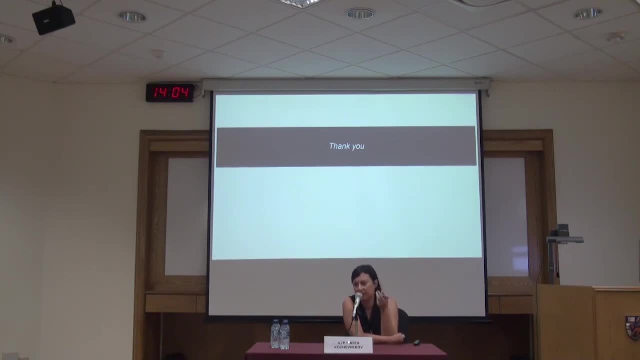 So trade-offs actually weren't even in five, six years old, Which actually is definitely due to genetic predisposition and genetics. Now the trade-offs start to deepen depending on what classes they take. So if they go into science track, the trade-off becomes even more obvious later during their studies. 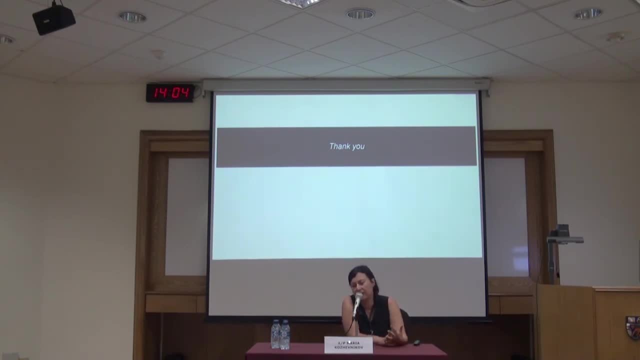 And about architects. architects is a very non-homogeneous group. Italian architects- they're more into object visualisation. They're actually all high in object visualisation, While American architects all high in spatial visualisation. So there's also kind of trade-off between them. 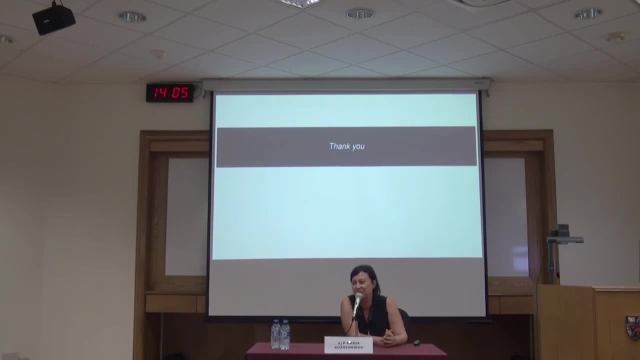 And they also self-report themselves as very high in both. But this is not actually the case. This is the only group who cannot report self-report objectively their object and spatial visualisation scores. Other group kind of. you know, they're not high in spatial, they're not high in object. 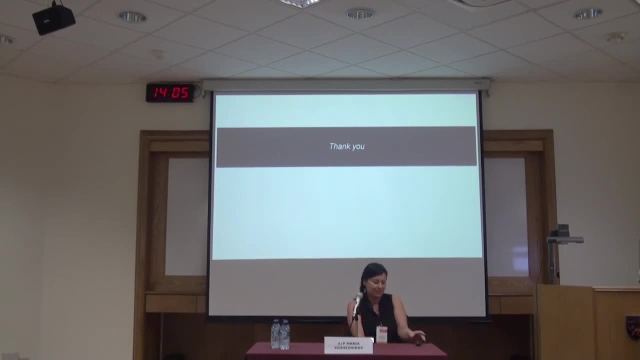 Any more questions? One over there. Hello, I'm Professor of Architecture, So I fall into your troublesome group And it seems that we are in trouble all the time in every university we work at, Because universities require our intake- the students, the cohorts that we take to actually score very high in sciences. 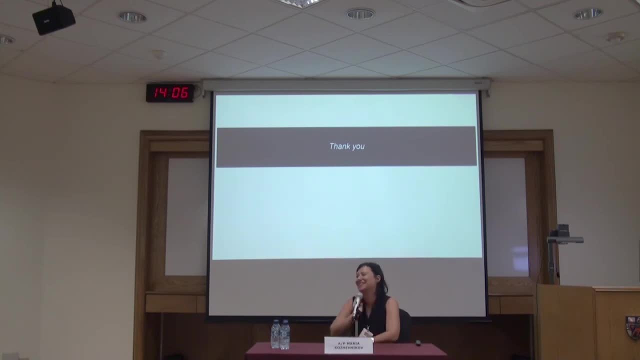 And then we are trying to teach them to score very high In a different category And that produces a lot of stress for students. We are infamous for producing those stress students. Who reposes on higher than everything? What are the chances of actually doing that within the five-year course? 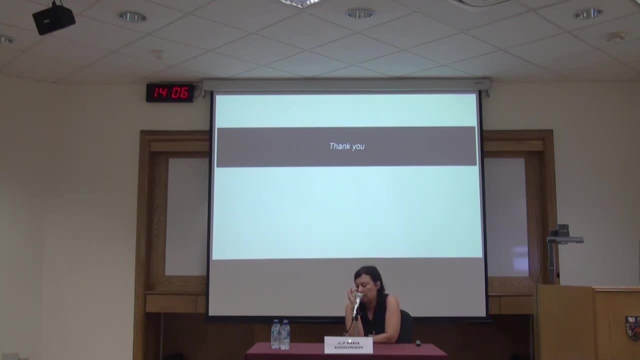 But that's again. I think it's because of these ideas that spatial ability and science is the most important in every domain, Which you know when I was in college In Italy. during the sabbatical They also have spatial visualisation workshop for artists there. 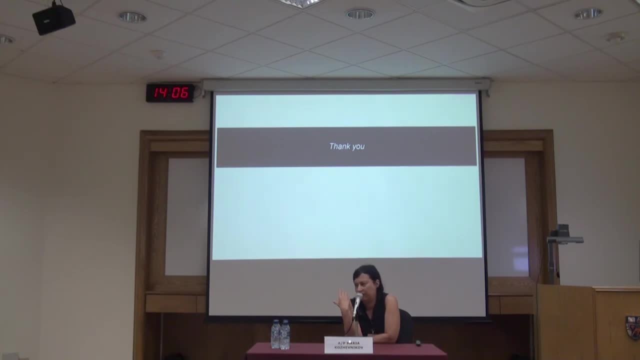 Venice Academy of Art And I was really surprised why Venice? you know artists need spatial visualisation workshops Because it's kind of, you know, it's good to increase the spatial visualisation. So this is what I'm really trying to show. 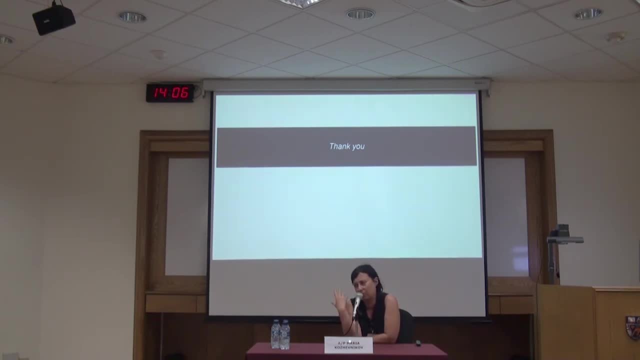 This research? this is not the case. Don't you know? don't do, don't train one, Maybe you can impede the other, which is no less important. Creativity for professional development. Yeah, Any more questions? I love the insight as well about the 2D versus 3D art. 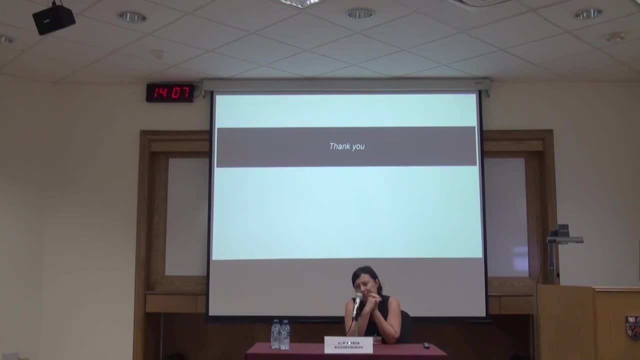 Where you have your sculptors, who seem to be doing the spatial visualisation, And your non-sculptors, who are doing what's referred to as object visualisation. I wonder if 2D and 3D is a better characterisation of the kind of visualisation skills that people have. 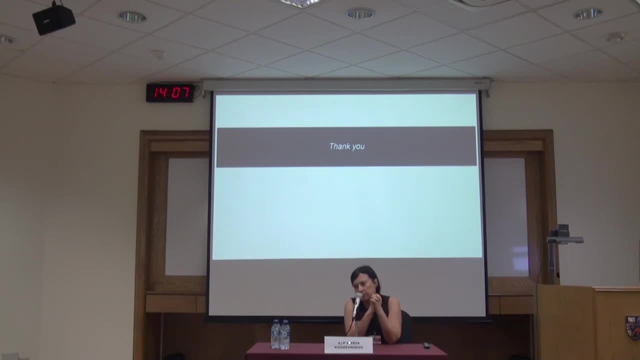 And again how that might tie into the cultural expertise that we have of watching TVs and reading books on flat media. So 3D is spatial visualisation. You know most especially when you need to manipulate images in 3D space. 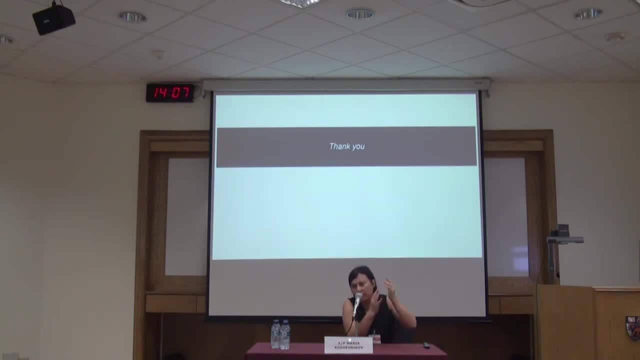 Object visualisers are not able to do it. So they're able maybe to imagine static 3D space, But it's not. it's not flexible in visual motivation. So 3D usually is spatial visualisation, But it's way more than just 3D, right. 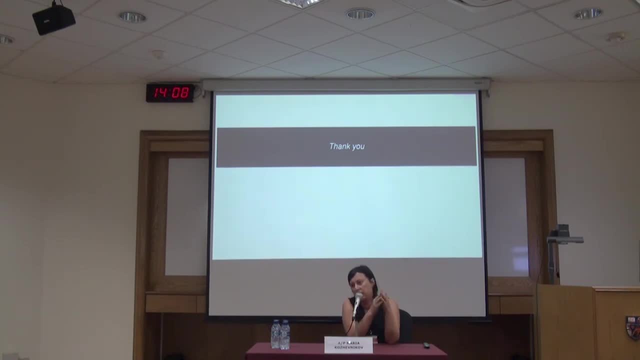 So people who could like in spatial visualisation, building schematic spatial images- they're usually better on 3D transformations. So people like object visualisers who could in shape and colour- they're usually not as great in 3D transformations. So sculptors are a really unique group. 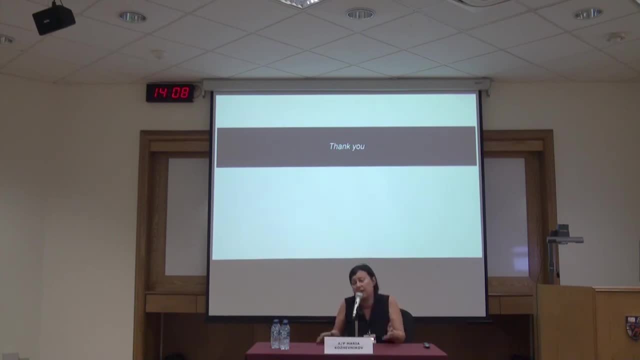 Somehow combined, at least shape and 3D, but not colour or texture and 3D. So they didn't have these skills. But I guess what I'm wondering is whether the neurological substrate is not about objects versus spaces, but two versus three dimensions. 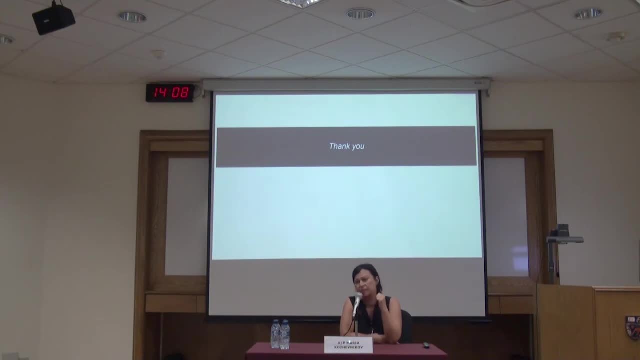 That's not exactly spatial manipulation. It's spatial, spatial pathway. 3D manipulation in 3D space is spatial. it's spatial processing pathway. It has nothing to do with object visualisation, Right Yeah? So to answer your question, 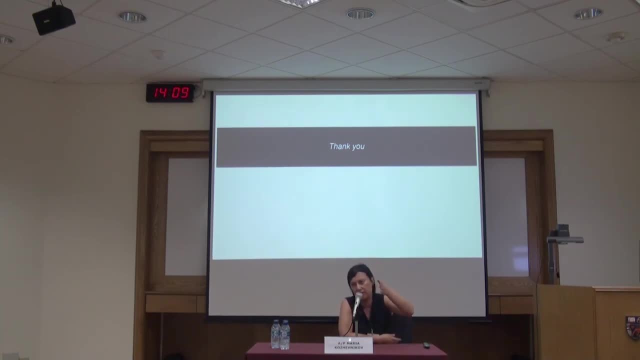 I mean 3D transformation happens in the spatial processing pathway, The same as colour transformation happens in object. Yeah, You need resources in spatial pathway to do 3D transformation in space. Okay, One question over here, Thank you. Creativity may have multiple aspects or dimensions. 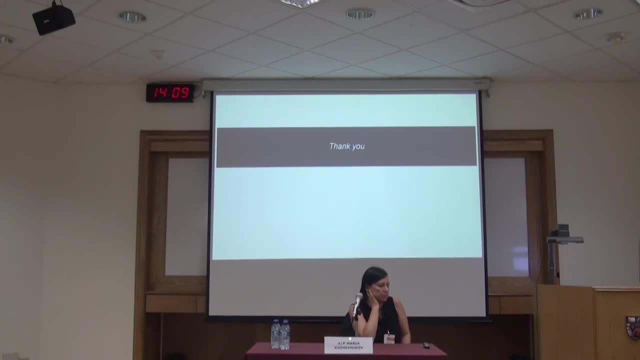 So we are curious: how do you measure or quantify creativity? How I measure creativity: Yeah, Okay. So for creativity we divided: okay, there are no good creativity tests, That's a problem. So for scientific creativity, to measure scientific creativity. 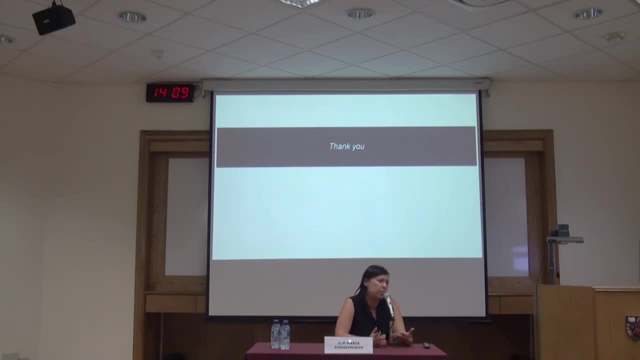 we usually ask these scientists to report the number of their papers and the status in the field And we also gave them inside problem solving questionnaire, which the exchanger showed here, Because this questionnaire inside problem solving showed actually to correlate with scientific profession. So this is how we measure inside problem solving questionnaire. 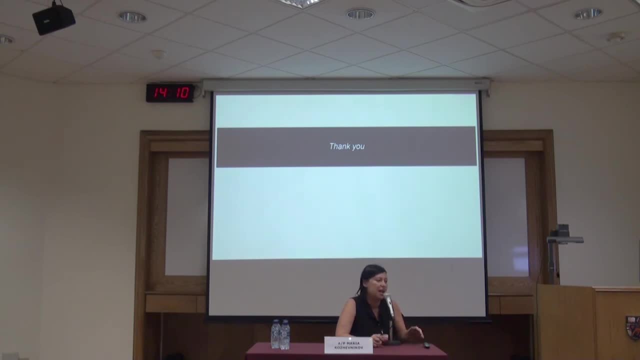 We measure spatial, we measure scientific creativity And for artistic creativity there is this test which I forgot its name. It's very famous but not very valid. It gives different objects and ask them to report and interpret what people see, So we use that one as well. 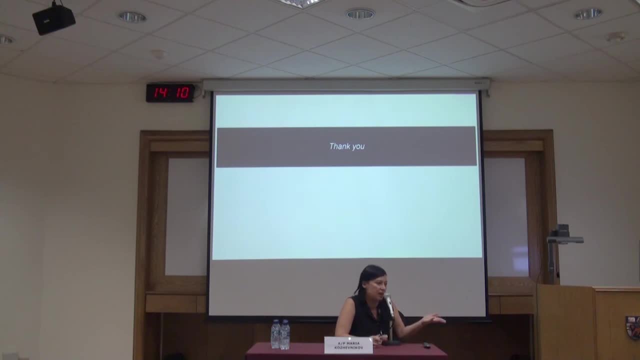 But mostly we base our data on self-reports Again: artists, how creative they seem in the field, how many pictures, galleries, exhibitions they have. So we actually want to self-report data on this. So the creativity is defined by each profession. 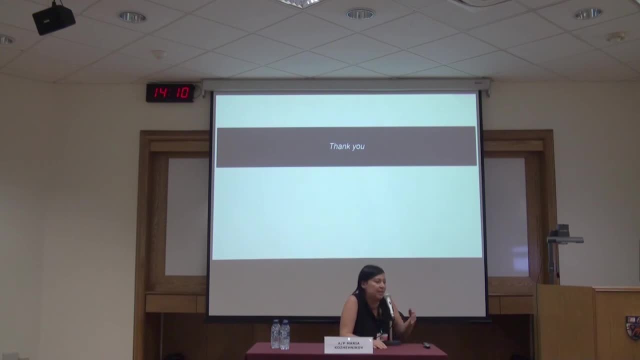 Yes, Very different. It's very different And it's very different again, cognitive components required to be creative in particular field. Thanks, Thank you. One question: Could you remind me what the brain areas have to do with spatial processing? 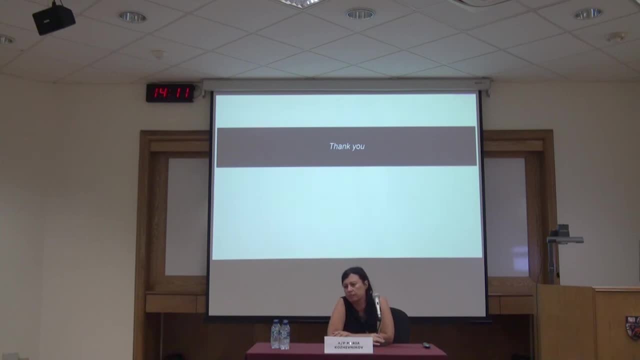 Sorry, I can't hear you. Could you remind me what the main areas have to do with spatial processing Brain areas? Yes, Okay, It's called dorsal brain areas, And does it also, because some of what we talked about is also spatial working memory as well. 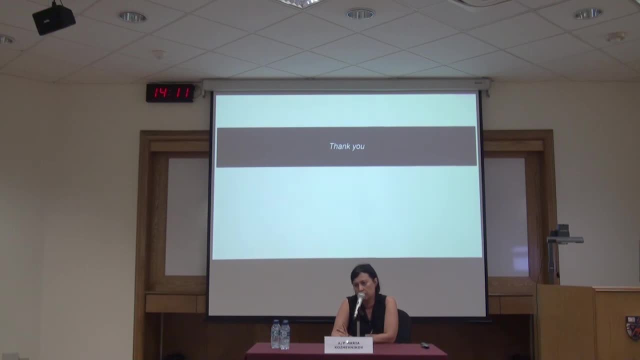 So just trying to remember this right, I think actually, things like that, the campus, both pathways. you don't expect it to be dorsal, No, no, no. Usually, you know, the cognitive maps create and give a compost information from parallel pathways and information. 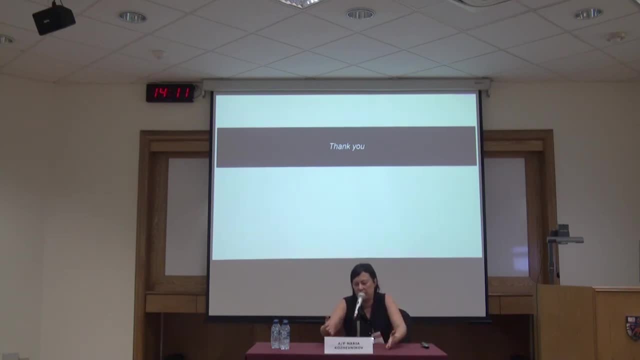 But here I'm talking really about. this is very famous: what and where? pathway, what is object appearances, where is temporal areas and where is spatial processing? When you showed your developmental graph, I was struck that you could kind of maybe overlay the. 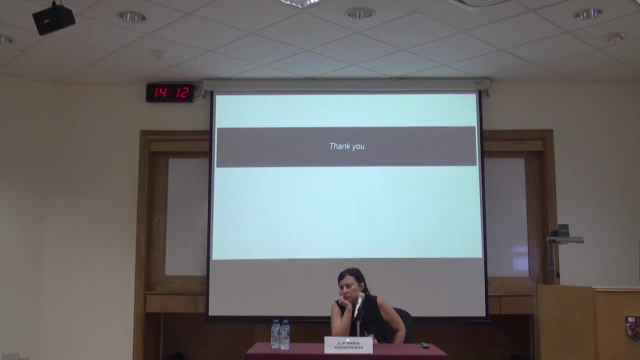 you could think about patterns of growth for the prefrontal vertex also increasing right with the object, with the ventral. But then I started thinking what might be going down? Okay, Going down. I just wanted to explain. it's not really going down. 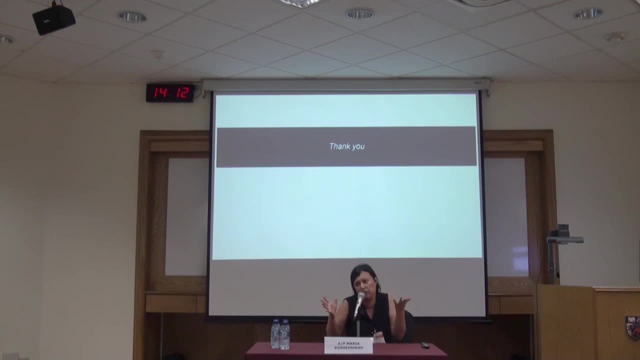 because it's for average in population, right? So if you look at average in population, it goes down. But I just want to say, I just want to give you an example- It doesn't go down if a person actively engaged. 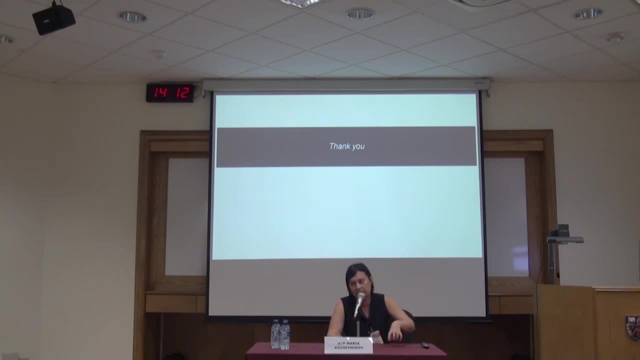 So, for example, a kid starts to do science very actively during critical period 14,, 16 years old, And if this person continues to do science, his or her spatial visualization will not decline with age, for example. You know, 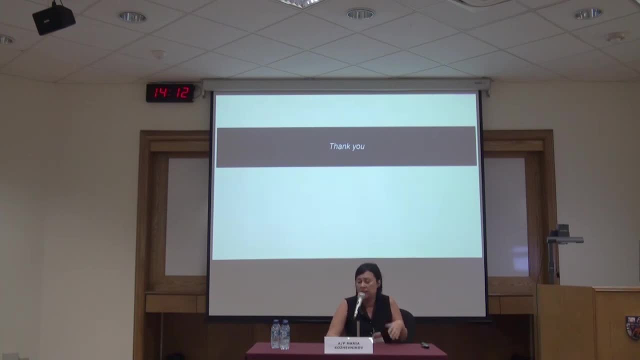 there was a study which shows that engineers and pilots after- actually after 60, there was a huge dip. So spatial visualization is practically disappearing. So not in engineers or pilots who actively engage Even 65 in their profession. actually stays the same from youth. 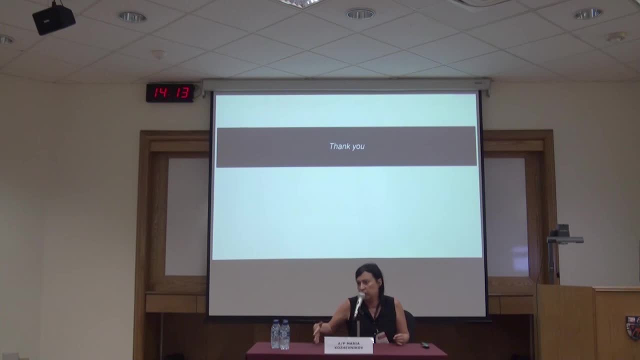 You know, until they get retired. after two months of retirement it quickly goes down. So the question is: as long as you're actively using it, it does not. there is no. there is no decline And memory for information. 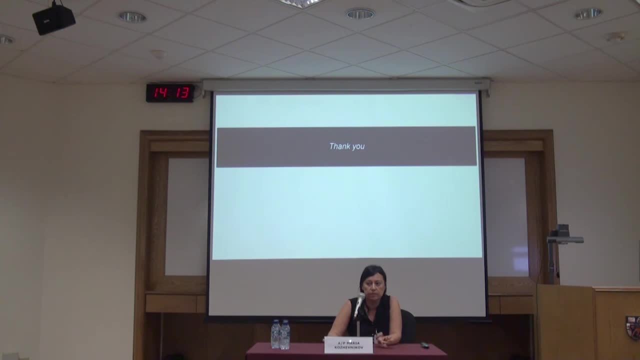 that's learned is it? is it influenced by which stream you're using to learn that information? Memory for object? learning is object. It's object passively, So it does not decline with age. It doesn't matter if you train it or not. 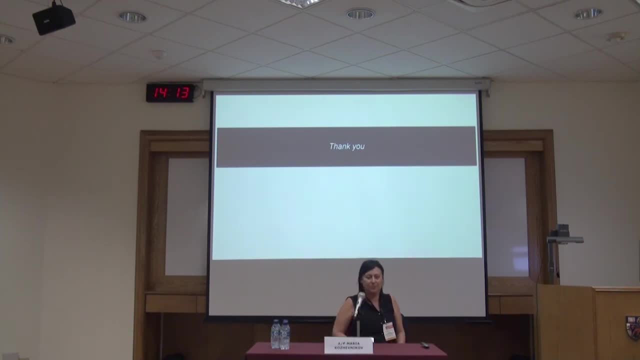 It actually goes on and on and on. All right, We won't go until next talk. Please join me in thanking Professor Kochenko.